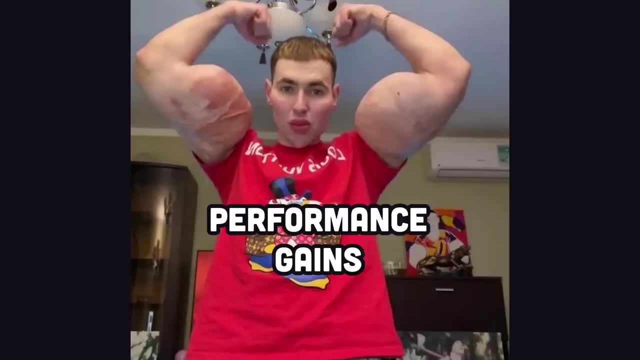 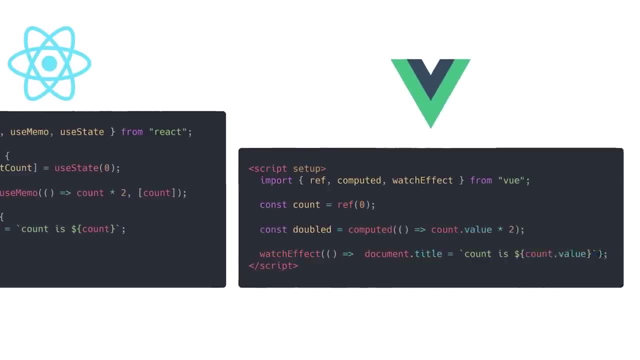 this compiler in production to power Instagram and will likely bring solid performance improvements. but, most importantly, it will simplify the code we write as developers. Currently, React code is pretty ridiculous compared to frameworks like Vue, Svelte and Solid. Like imagine, we have some state that needs to be computed into another value. 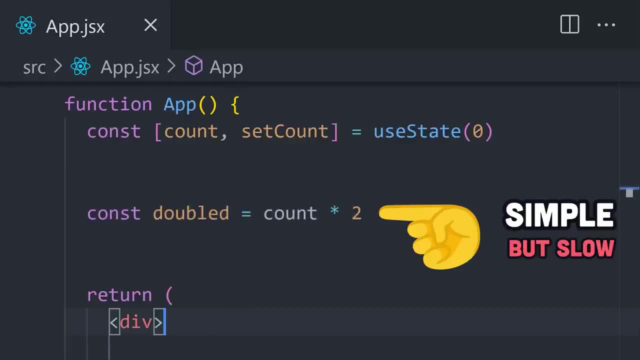 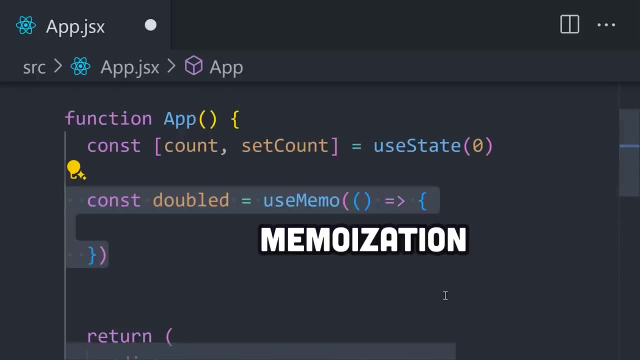 We can do it like this in React, but that value will be unnecessarily recomputed every time the component re-renders. It's inefficient To address this. React provides a hook called useMemo. Memo means memoization, which itself means remember. It wraps the computation in. 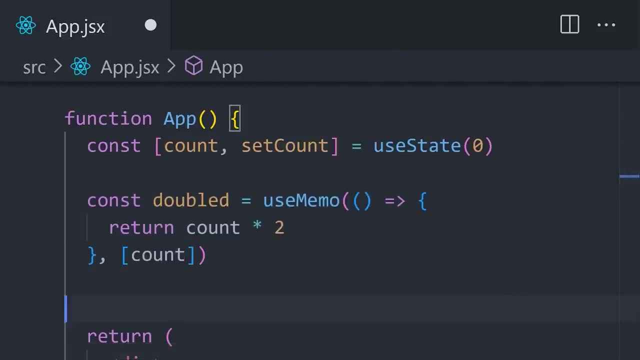 another function which will only run when the state that it's dependent on changes, which has to be explicitly put in this array. If we look at all the other frameworks, though, they don't do stuff like this. If we look at the other frameworks, though, they don't do stuff like 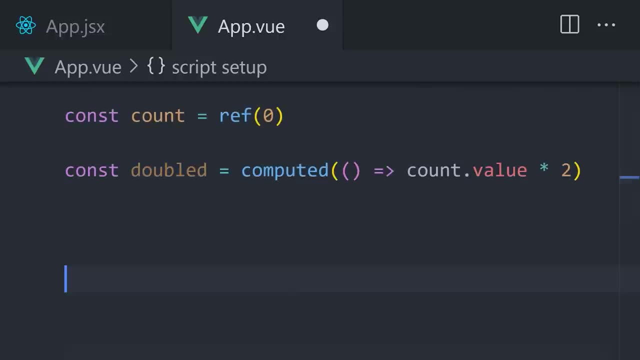 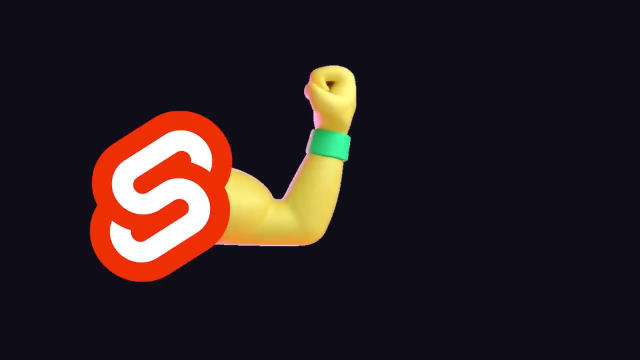 this, Like in Vue, we have this computed function, but there's no need to include that dependency array. And in Svelte 3, it's even more simple with the dollar sign syntax, although it's being replaced with a rune in Svelte 5.. The reason: these frameworks can let you write more simplified. 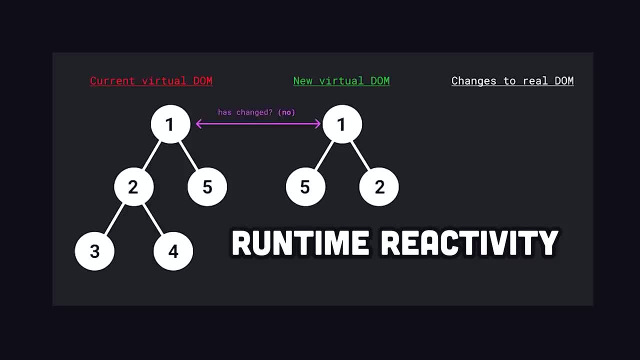 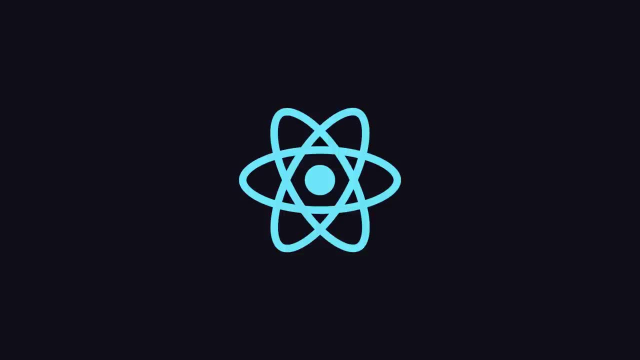 code is because they have a compiler, unlike React, which is purely runtime-based. They look at your code in advance to figure out where the reactivity is and bundle that into the final product that goes to the browser. But now that React is getting its own compiler, it means hooks. 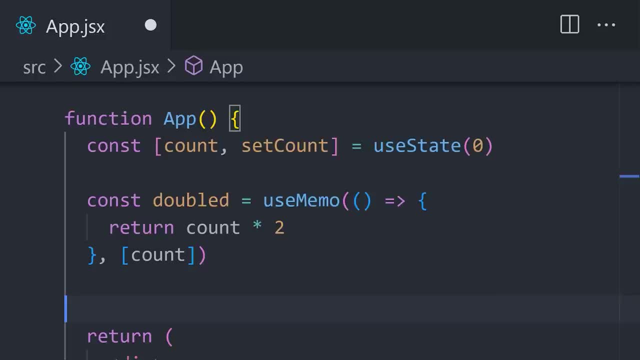 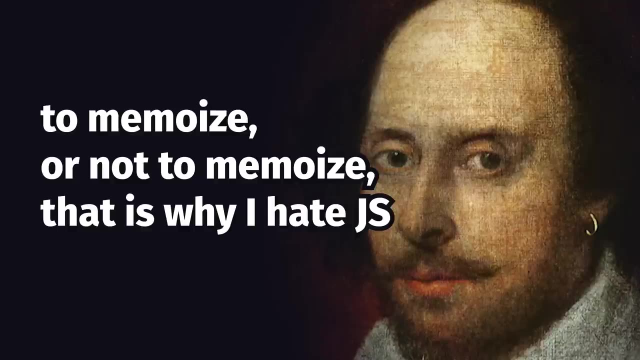 like useMemo and useCallback are a thing of the past, And that's huge because not only is the code as hell, but it also removes the mental boilerplate of asking the question to memoize or not to memoize. And they confirmed my conspiracy theory that React intentionally adds bad APIs like 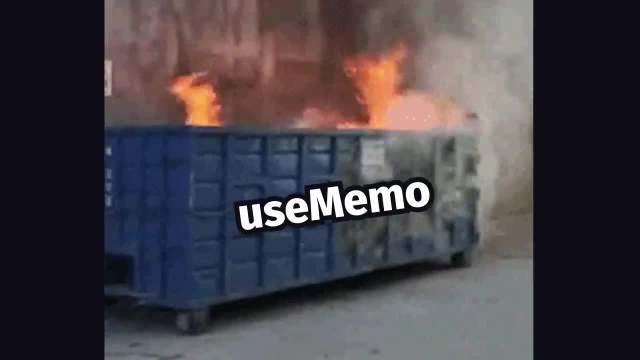 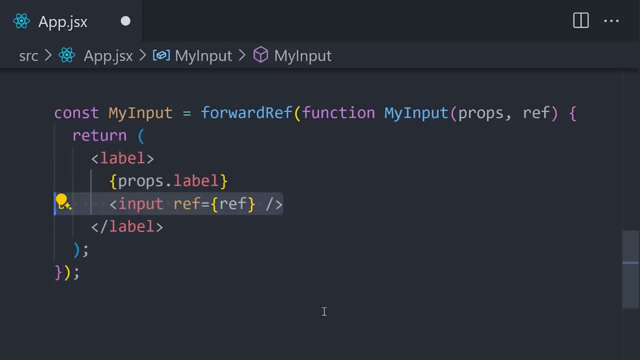 this just to look like geniuses when they remove them later on. But useMemo is not the only bad feature going away. Another thing you won't need in the future is forwardRef, which creates a higher order component when you need to expose a DOM node to the parent. Instead, ref will just be. 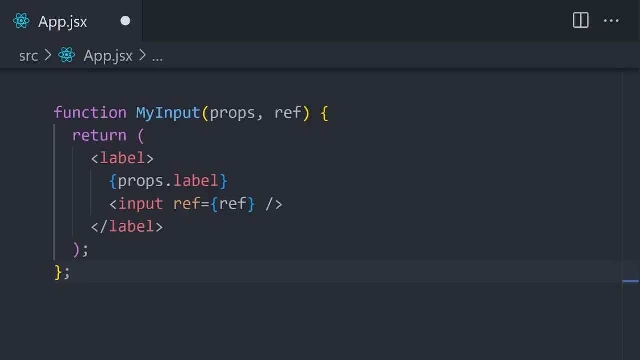 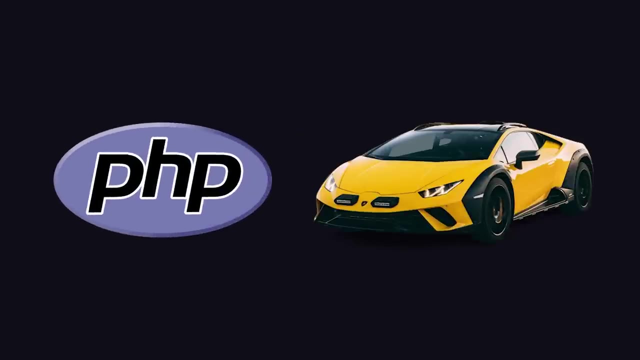 a prop so you can easily access it without having to wrap another function. That's an easy win, but a more controversial feature is server actions. You can already use actions in Nextjs, and many have described the developer experience as being like PHP. but 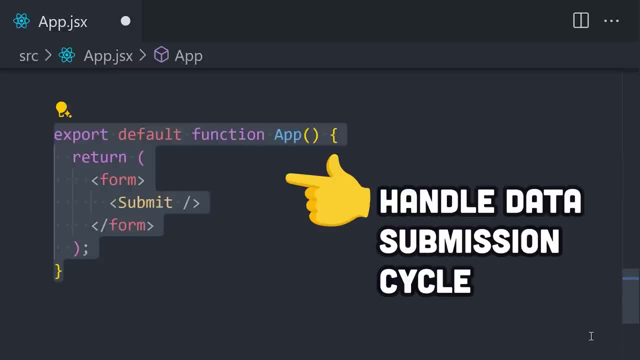 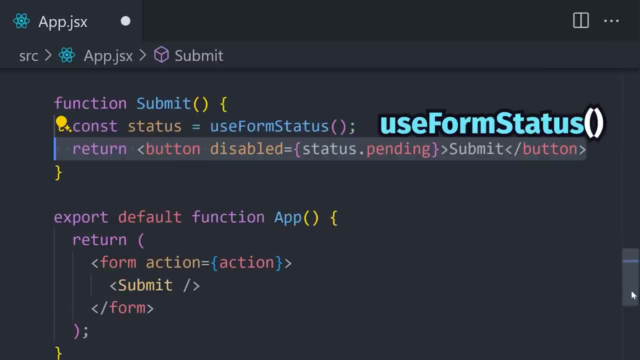 without Lambos. The general idea, though, is that React handles the data submission cycle for you from client to server and then back again. What's cool about this is React provides hooks like useFormStatus or useFormState to easily handle the data in a form, but then, alongside that,